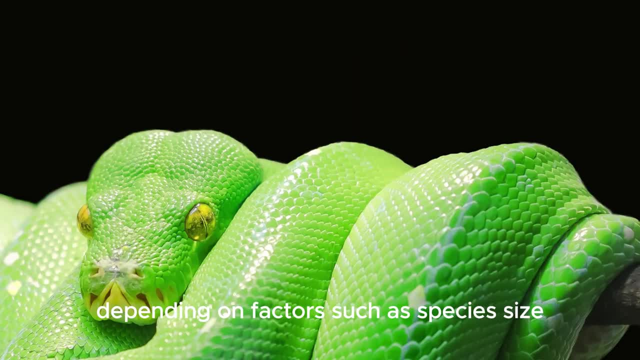 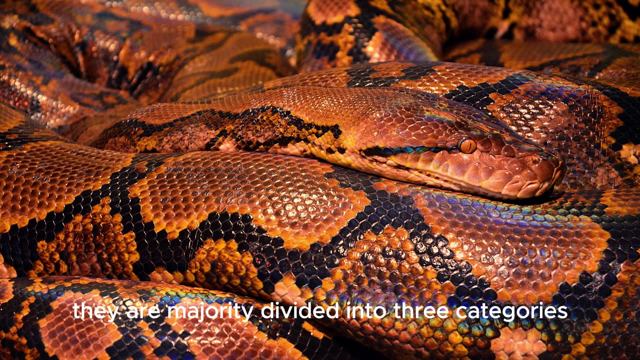 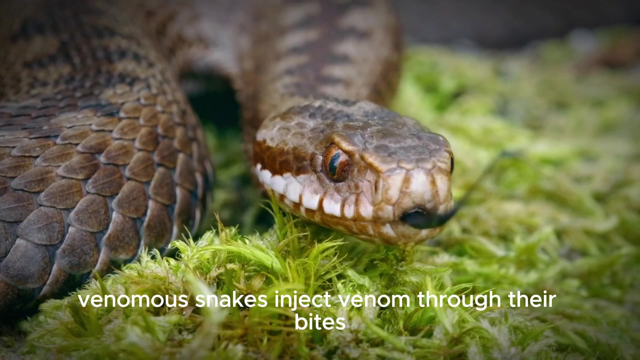 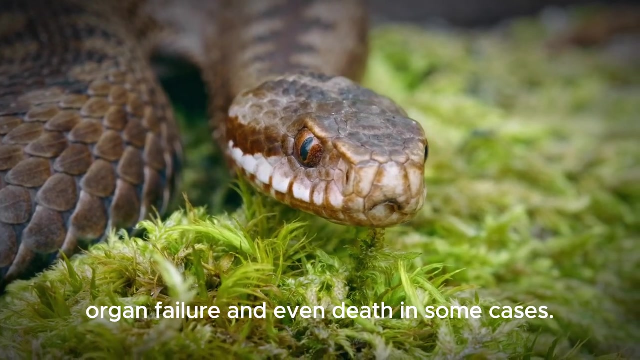 by snakes varies greatly depending on factors such as species, size, venom potency and the circumstances of encounter. They are majorly divided into three categories: 1. Venomous snakes. Venomous snakes inject venom through their bites, which can cause various effects ranging from mild discomfort to severe tissue damage, organ failure and. 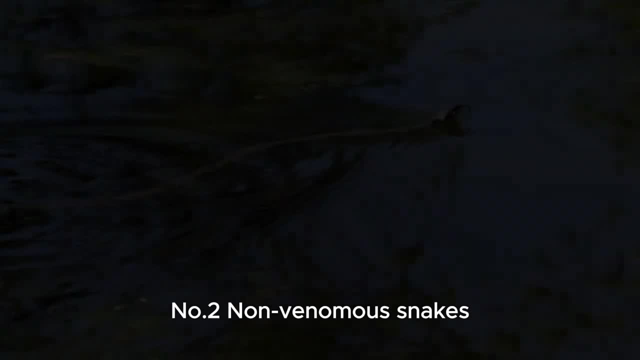 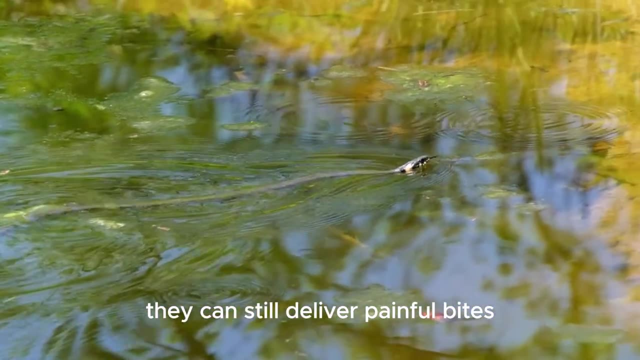 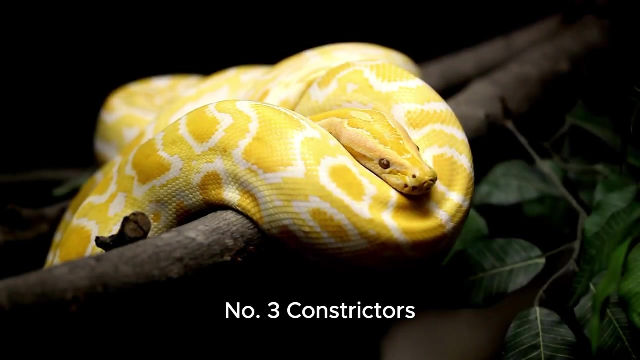 even death in some cases. 2. Non-venomous snakes. While non-venomous snake is lack venom, they can still deliver painful bites and some may carry bacteria. 3. Constrictors: Large constrictor snakes like pythons and anacondas can be dangerous. 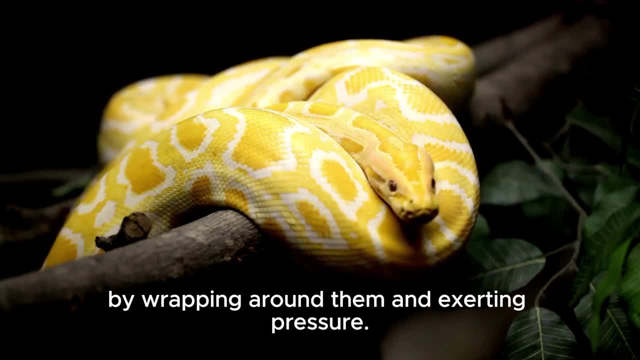 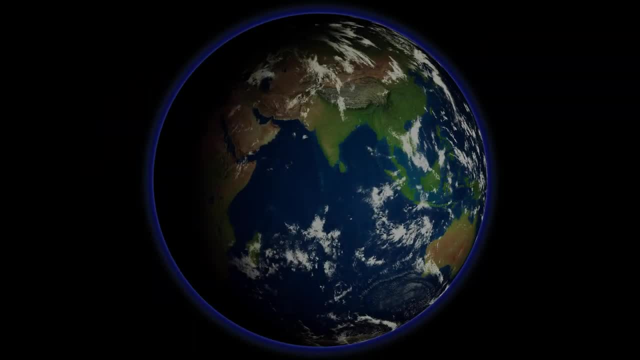 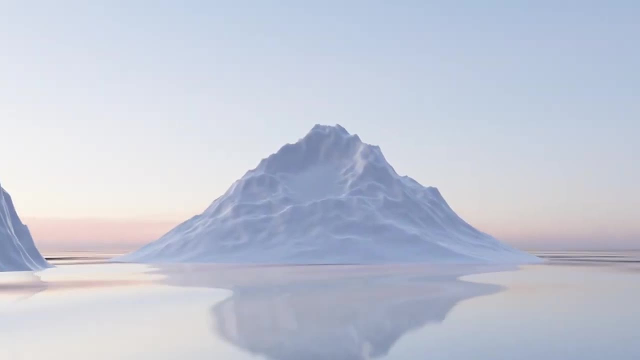 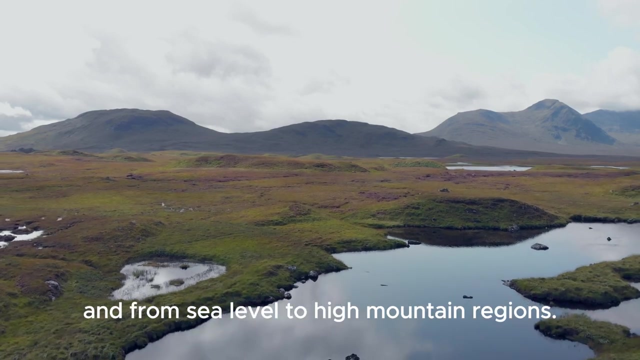 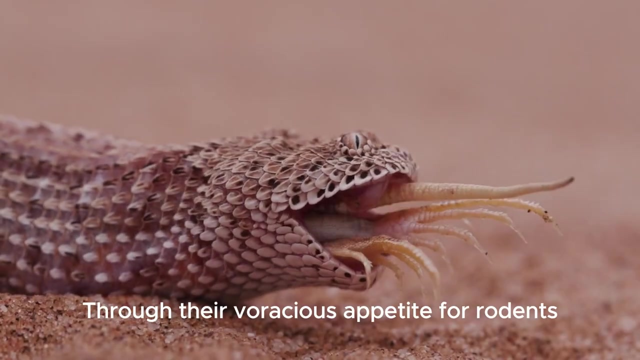 due to their ability to suffocate prey by wrapping around them and exerting pressure. Snakes are found on every continent except Antarctica, thriving in various habitats from deserts to rainforests and from sea level to high mountain regions. Through their voracious appetite for rodents, insects and small mammals, snakes serve as 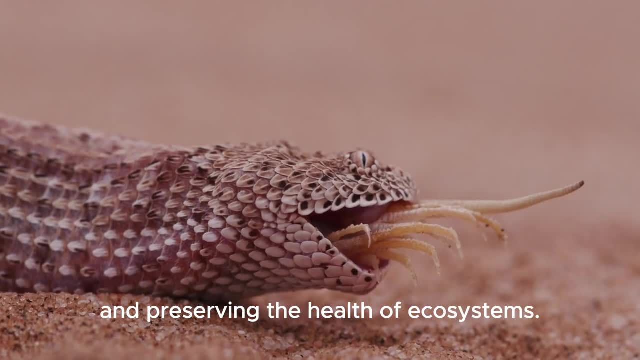 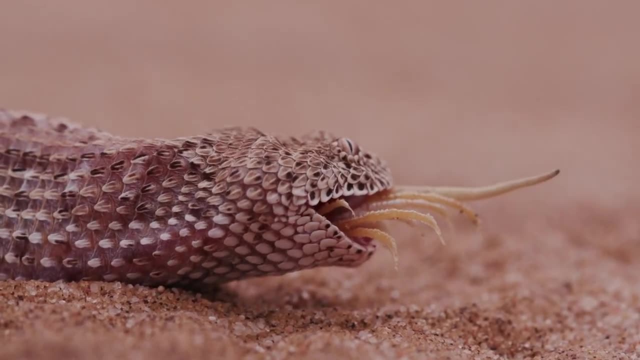 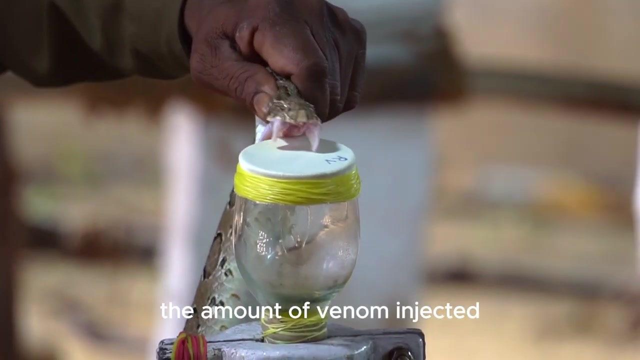 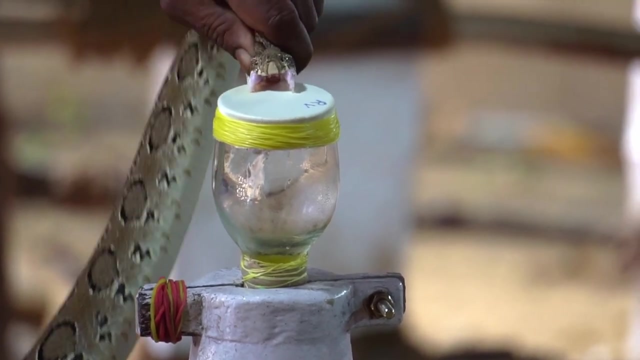 nature's pest control, preventing overpopulation and preserving the health of ecosystems. 4. Snake bites. Snake bites can be a serious medical emergency, depending on the snake species, the amount of venom injected and the location of the bite on the body. 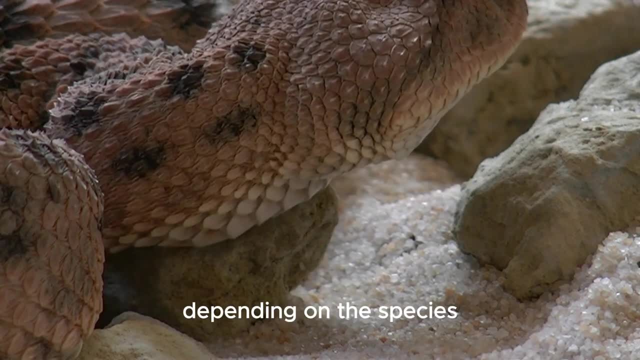 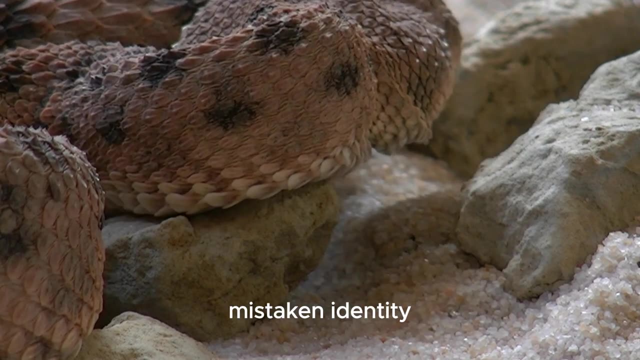 Snakes may bite for several reasons, depending on the species and the circumstances of the encounter: Defense, protection of territory or young, mistaken identity, hunger, illness or injury, handling, stress. 5. The bite, The biting force of a snake can be a serious medical emergency, depending on. 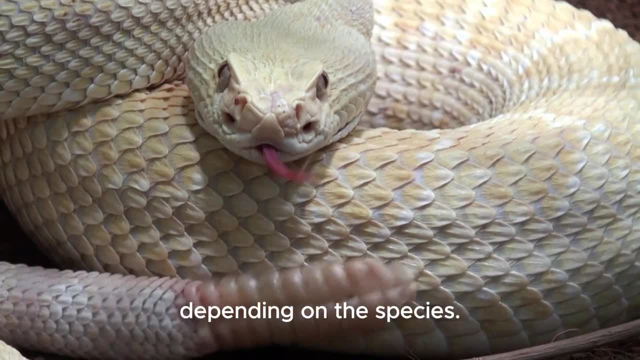 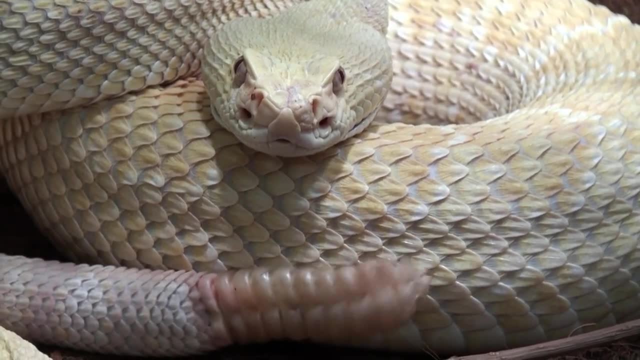 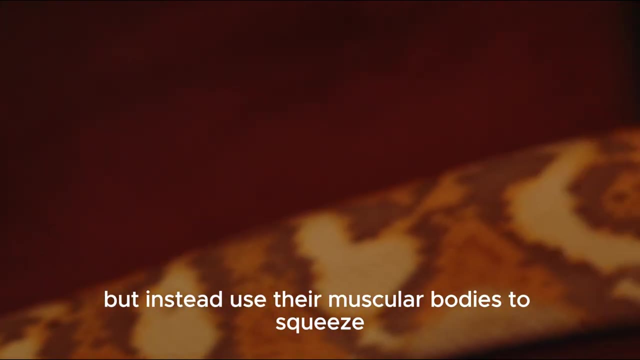 the snake species, the amount of venom injected and the location of the bite on the body. The bite force of a snake can vary widely depending on the species. Generally, larger snakes with larger heads and stronger jaw muscles will have more powerful bites. For example, constrictors such as pythons and boas do not possess venom but instead. 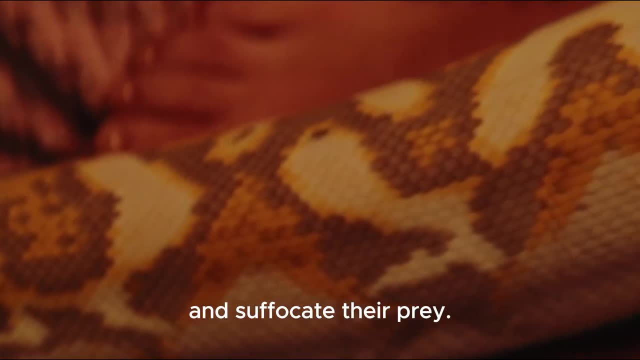 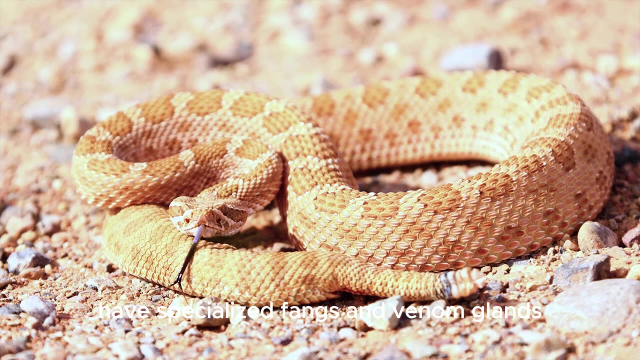 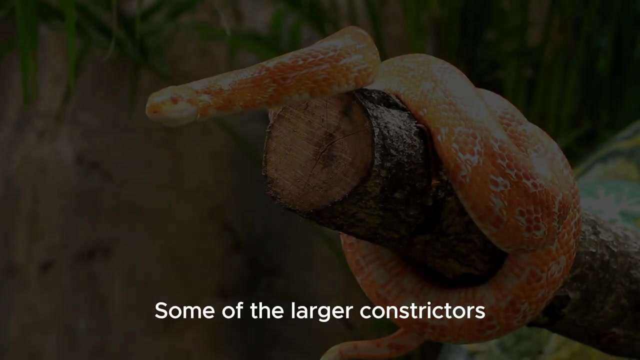 use their muscular bodies to squeeze and suffocate their prey. In contrast, venomous snakes like vipers and cobras have specialized fangs and venom glands to inject venom into their prey or as a defense mechanism. Some of the larger constrictors, like pythons and anacondas, are capable of delivering bites. 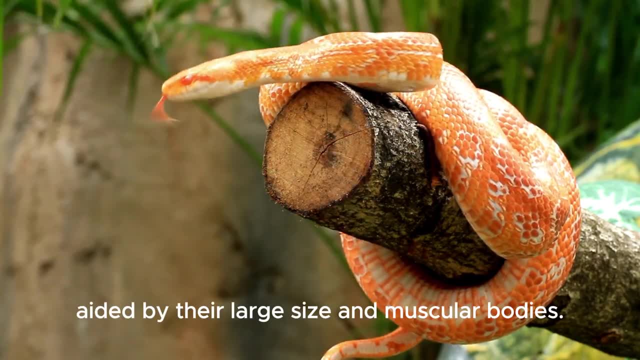 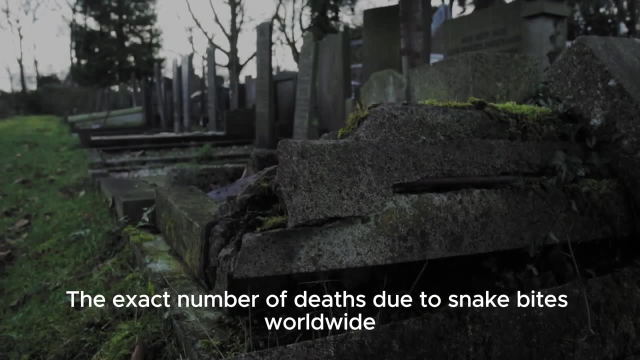 with considerable force, aided by their large size and muscular bodies. The exact number of deaths due to snake bites worldwide can vary from year to year and region to region. According to the World Health Organization, the number of deaths may vary from year to year and region to region. 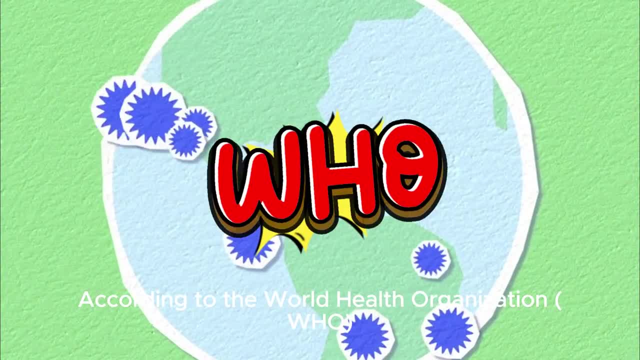 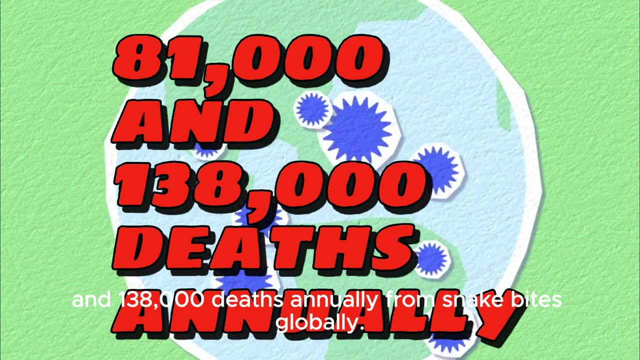 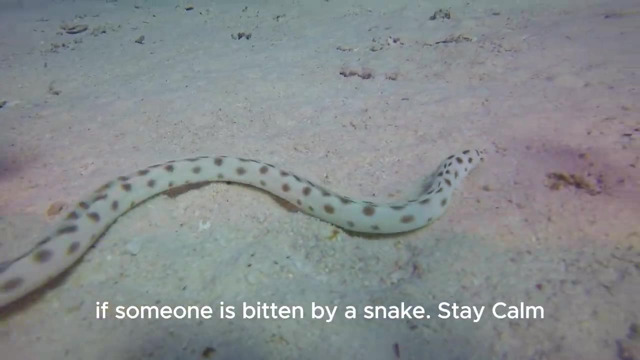 According to the World Health Organization, the number of deaths due to snake bites worldwide can vary from year to year and region to region. It is estimated that there are between 81,000 and 138,000 deaths annually from snake bites globally. Here are some general steps to take if someone is bitten by a snake. 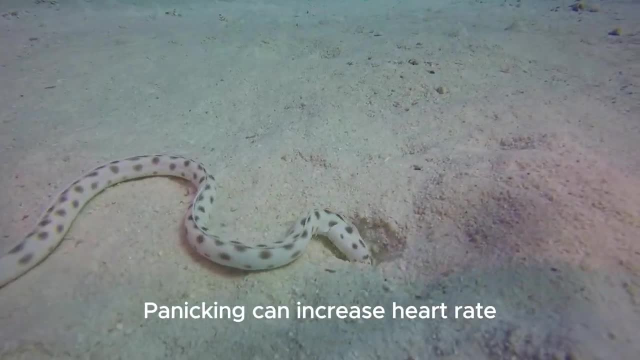 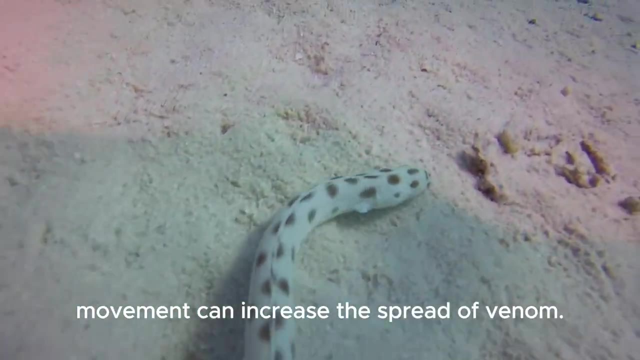 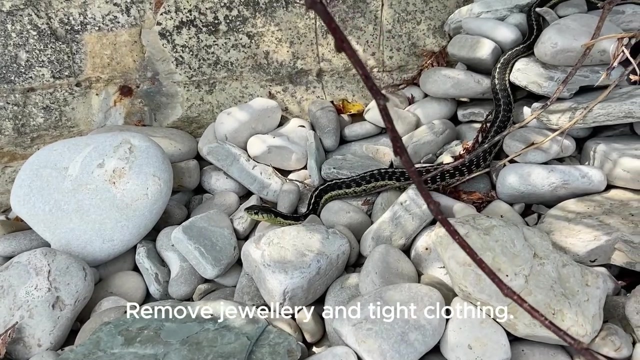 Stay calm. Panicking can increase heart rate and spread venom faster through the body. Keep the person still. Movement can increase the spread of venom. Encourage the person to lie down with the bite area closed. Stay calm. Keep the bite area lower than the heart if possible. 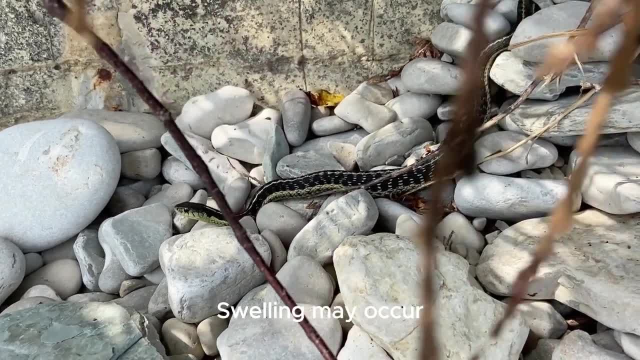 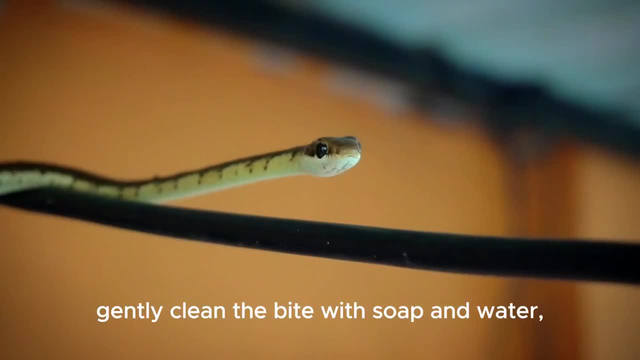 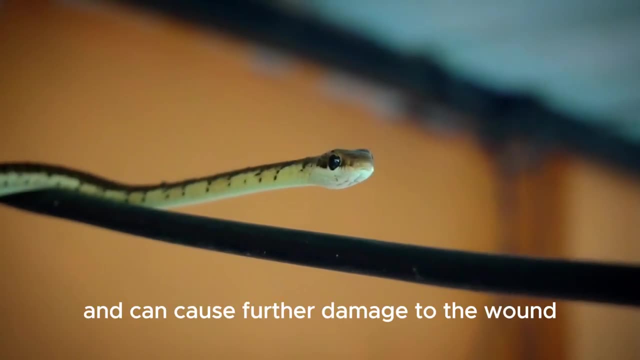 Remove jewelry and tight clothing. Swelling may occur, so it is essential to remove anything that could constrict blood flow. Clean the bite area Gently. clean the bite with soap and water if available. Do not attempt to suck out venom. This is ineffective and can cause further damage to the wound. 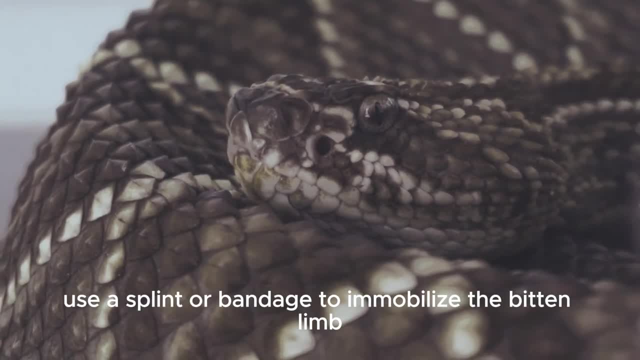 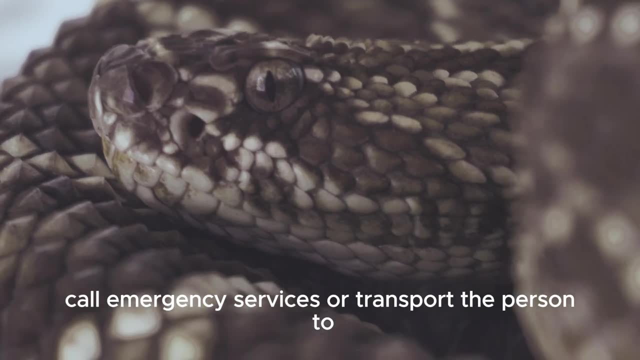 Keep the bite immobilized. Use a splint or bandage to immobilize the bitten limb if possible. Stay calm, See the patient, Hold the patient's hand to the side, keep them in a closed environment and try to make sure they are completely clean. 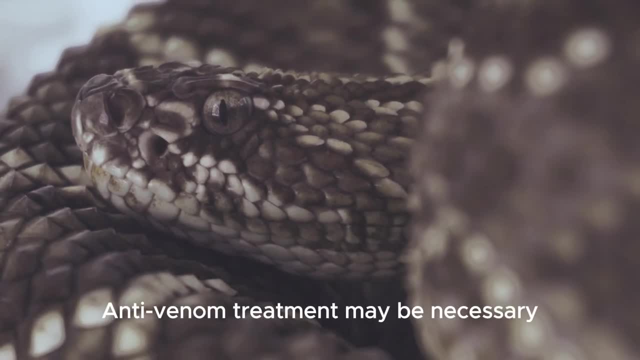 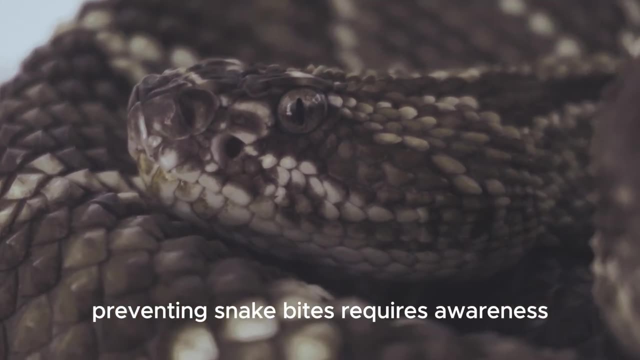 Stay calm, Call emergency services or transport the person to the nearest medical facility as soon as possible. Anti-venom treatment may be necessary depending on the type of snake and severity of the bite. Preventing snake bites requires awareness, caution and understanding of snake behavior. 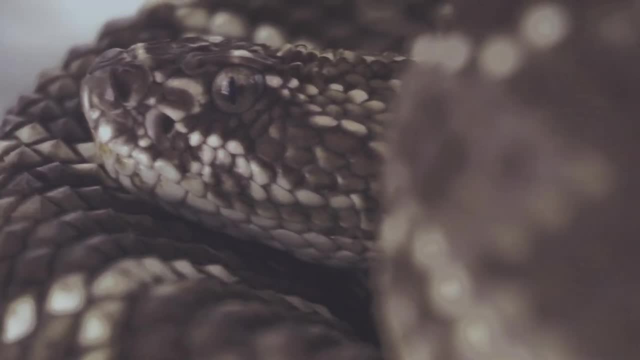 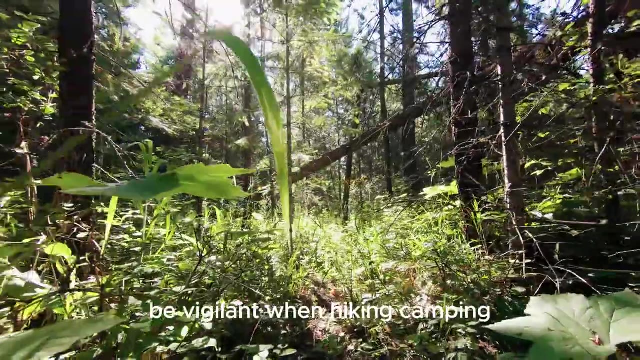 Here are some tips to help prevent snake bites: 1. everlasting its strong, vigorous and gentle bite. 2. keep the teeth open. 3. keep the body cool when it is bitten. Be vigilant when hiking, camping or working in areas where snakes are known to inhabit. 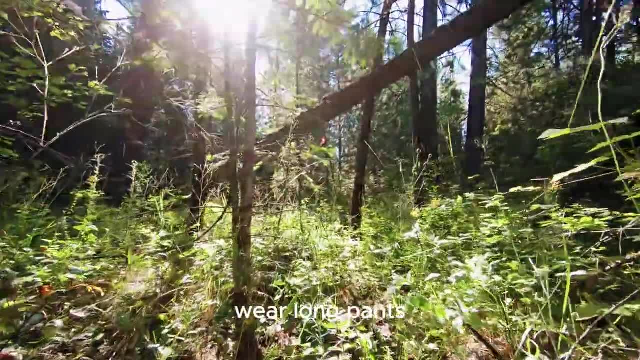 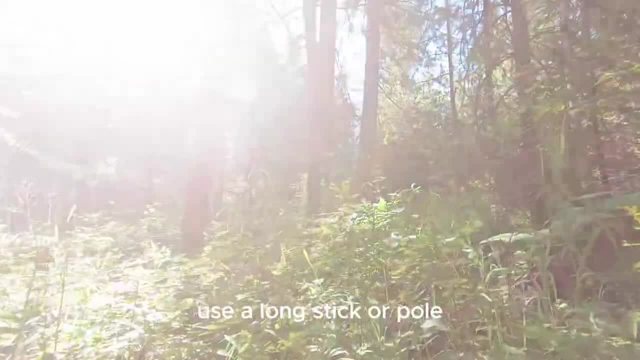 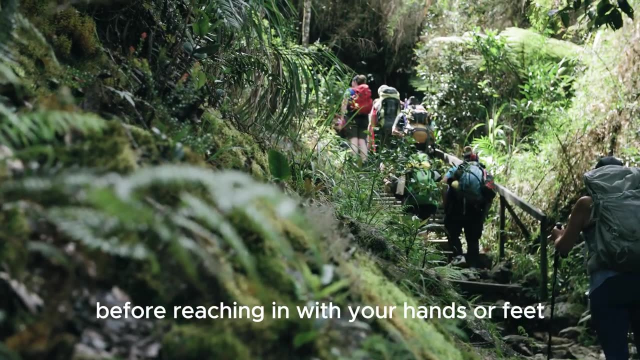 When in snake-prone areas, wear long pants, thick socks and sturdy boots or closed-toe shoes to reduce the risk of snake bites. Use a long stick or pole to probe areas where you cannot see clearly, such as tall grass or rocky crevices, before reaching in with your hands or feet. 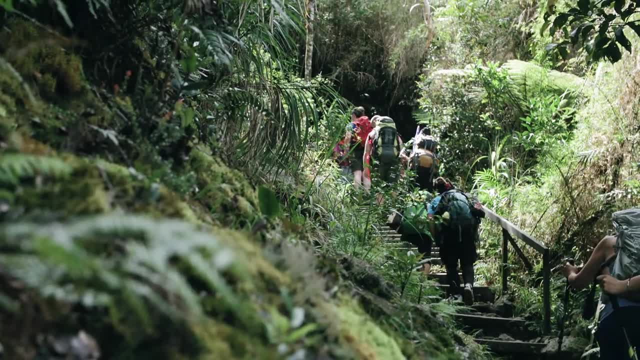 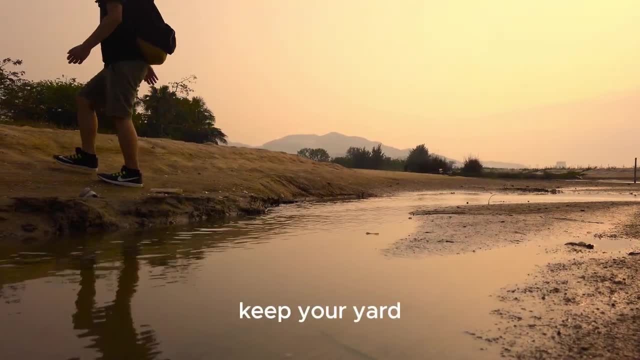 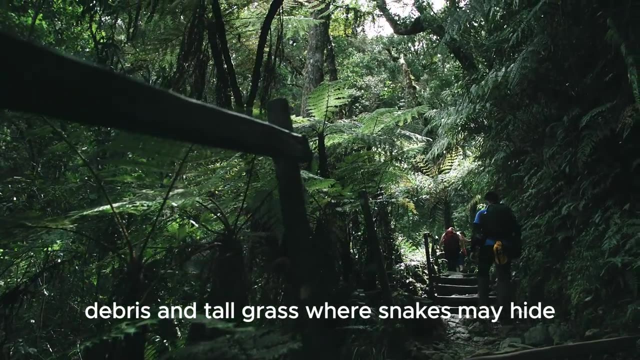 Be mindful around water sources. Snakes are often found near water sources such as rivers, lakes, ponds and marshes. Keep your yard, garden and outdoor living spaces free of clutter, debris and tall grass where snakes may hide. Store firewood, compost piles and other potential snake habitats away from your home. 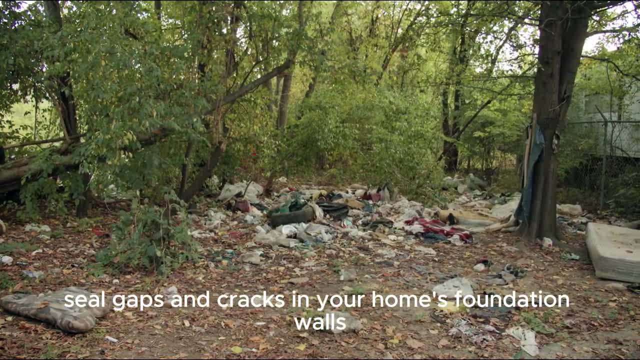 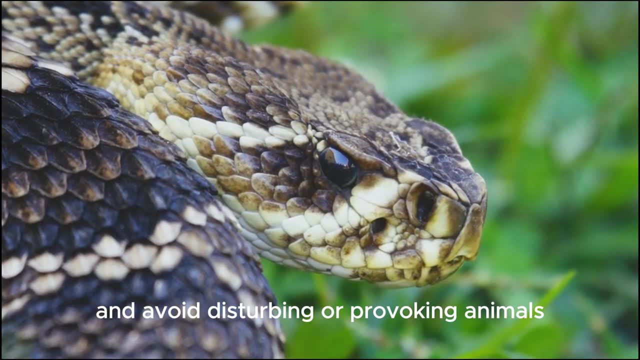 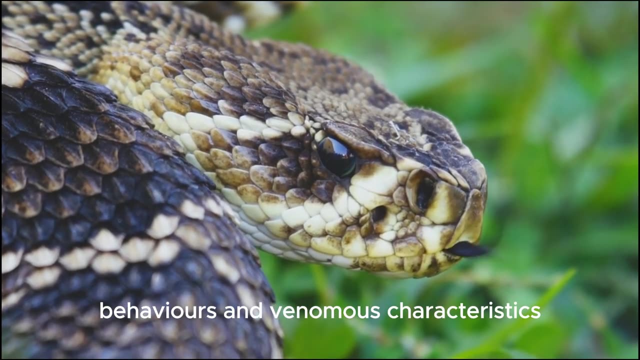 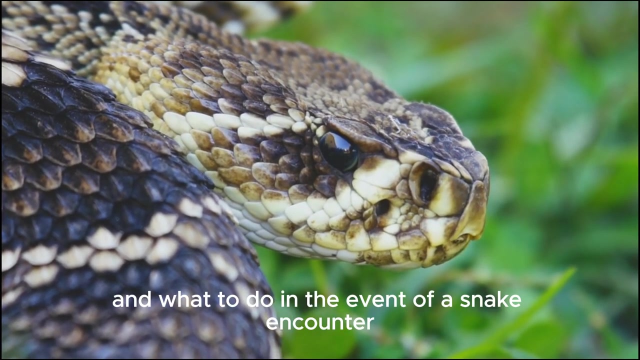 Seal gaps and cracks in your home's foundation walls and doors to prevent snakes from entering your home. Keep a safe distance and avoid disturbing or provoking animals. Learn to identify local snake species and their habitats, behaviours and venomous characteristics. Educate others, especially children, about snake safety and what to do in the event of a snake encounter. 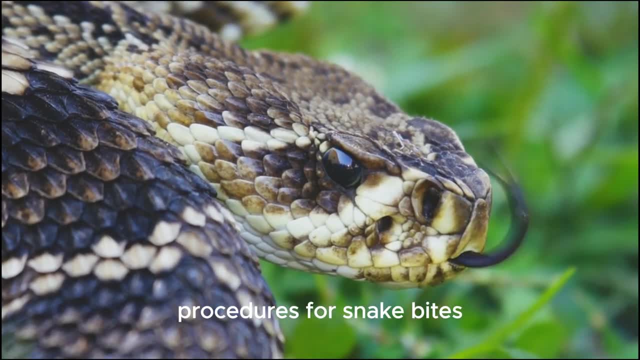 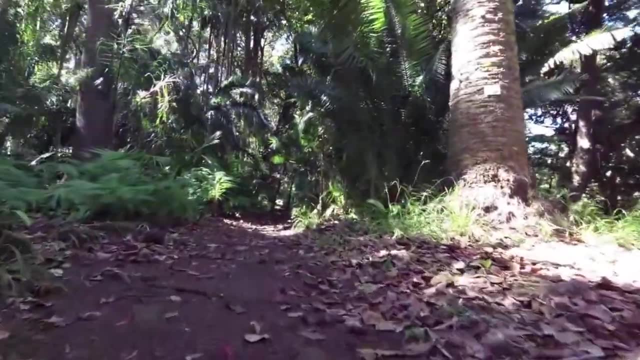 Familiarise yourself with first aid procedures for snake bites and seek medical attention immediately if bitten. By following these precautions and being careful, you can avoid snake bites. By being aware of your surroundings, you can reduce the risk of snake bites and enjoy outdoor activities safely. 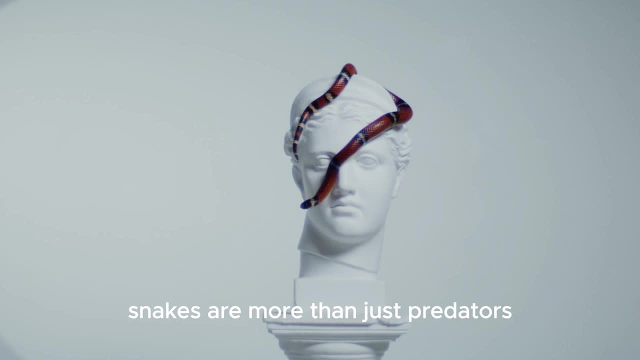 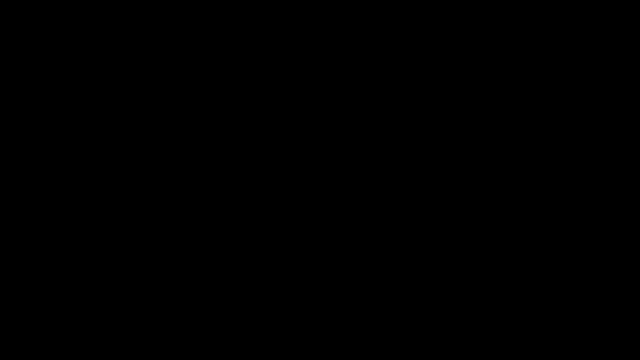 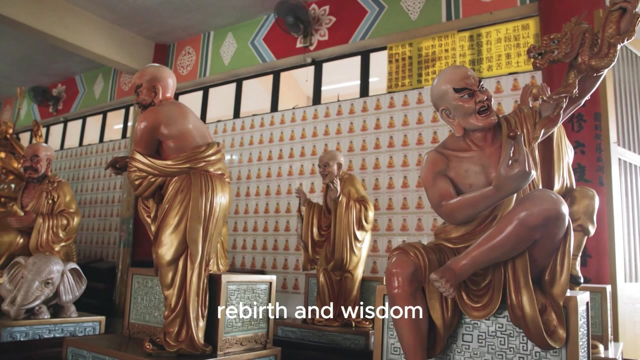 Take a look at snake-human relationships. Snakes are more than just predators. They hold cultural and symbolic significance in societies around the world. From ancient mythology to modern folklore, snakes have been revered as symbols of fertility, rebirth and wisdom, enriching human culture with their mystique and beauty. 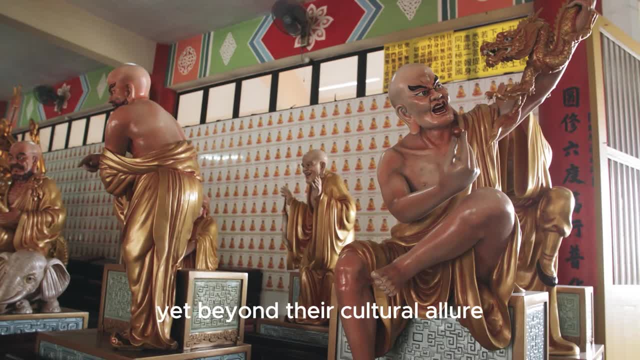 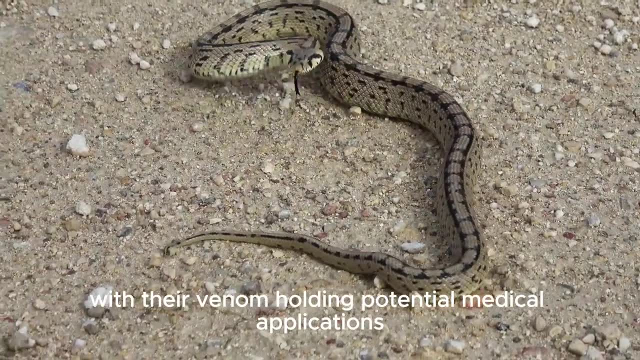 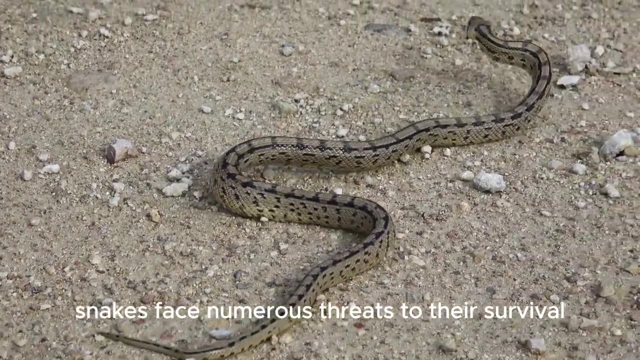 Snakes are also known for their beauty and symbolism. Yet beyond their cultural allure, snakes are subjects of scientific fascination, with their venom-holding potential medical applications. But amidst the wonder and awe lies a sobering reality: Snakes face numerous threats to their survival. 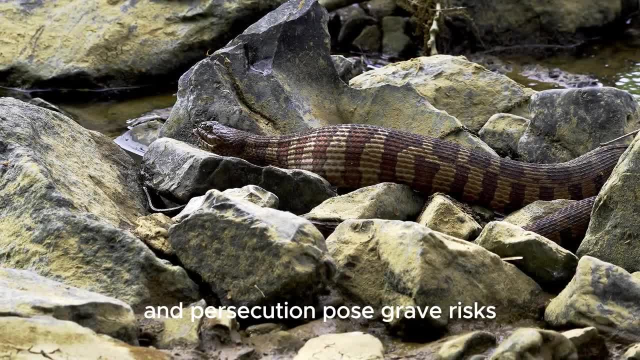 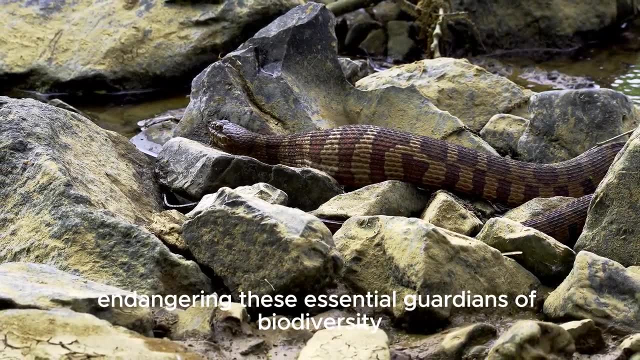 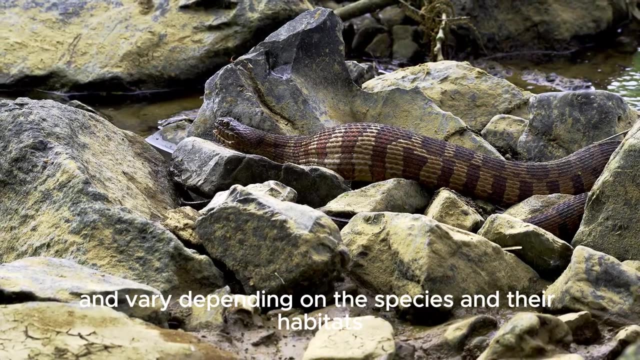 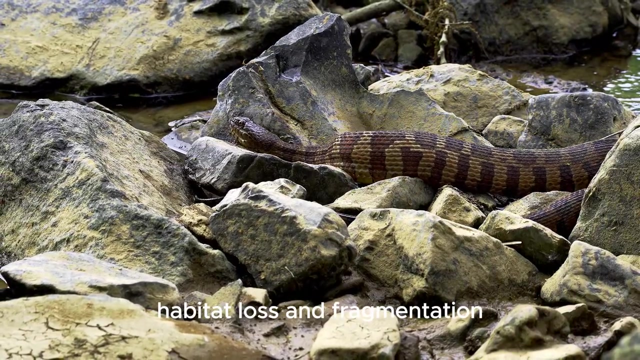 Habitat loss, illegal wildlife trade and persecution pose grave risks to snake populations worldwide, endangering these essential guardians of biodiversity. Conservation challenges facing snakes are multifaceted and vary depending on the species and their habitats. Some of the significant conservation challenges include Habitat loss and fragmentation.